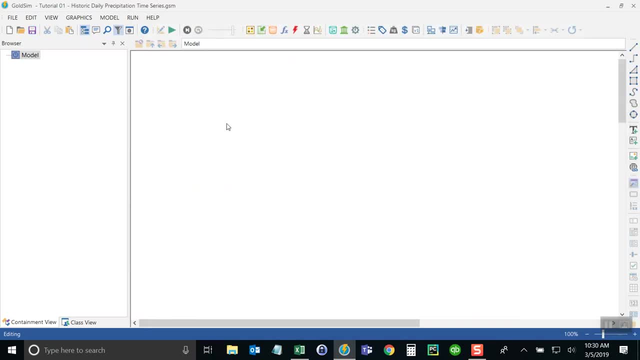 on my desktop here now I'll go and go ahead and create a time series element, and that's done by clicking on the inputs category button up here in the toolbar and then selecting time series. put that here and I'll call this precipitation underscore TS for time series and then I'm going. 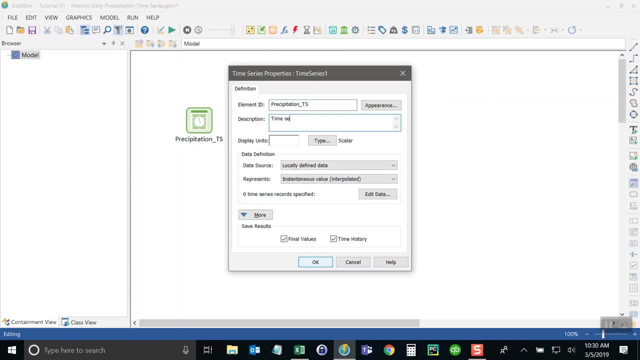 to describe it here: time series of daily average, and this just happens to be 1948 through 2018. okay, and my units are, on average, millimeters. millimeters per day. that's the daily average rate. millimeters per day. okay, I want to keep all of. 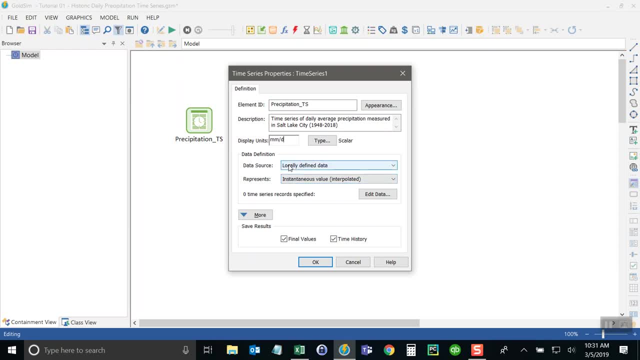 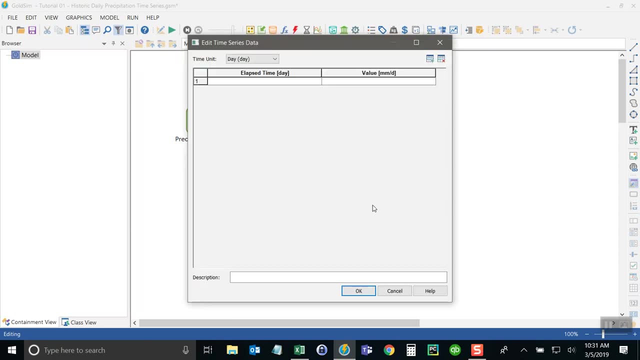 these the data definition settings the same. just use the default and then to paste the records in here, I'll go it here and click on edit data and what you'll see by default- the any goals and model is set up to run for an elapsed time, not a calendar basis, but eventually. 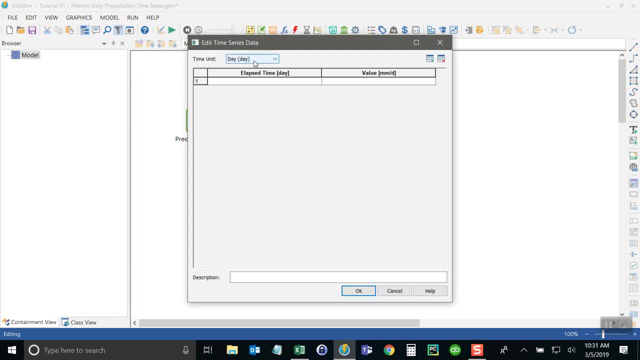 we're going to change that to run on a calendar basis but because it's set up to run for just an elapsed time with daily time steps, the time unit shown here for the the records are the. the daytime records is currently number of elapsed days, but I want to change that to calendar time. note that if we set up 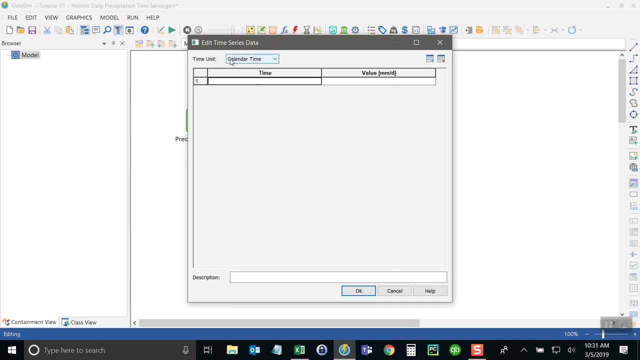 our model to be a count on a calendar basis. the default setting here would already be calendar time and you wouldn't have to worry about it. but I just want to make sure that that's set up for calendar time, because the values I'm going to be entering in here will be daytime or date format and they won't be. 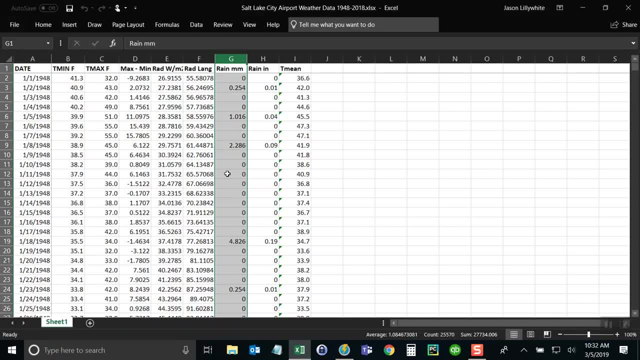 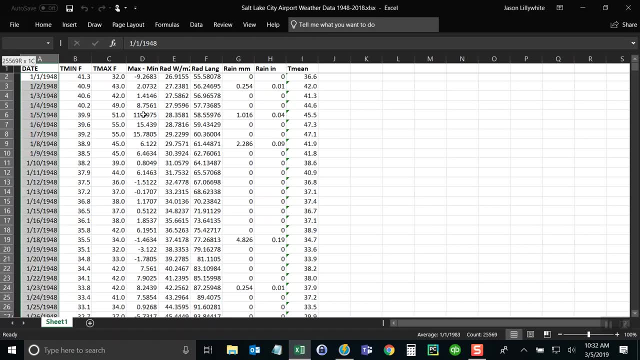 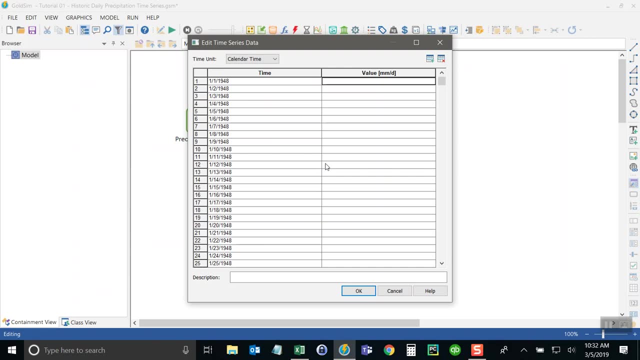 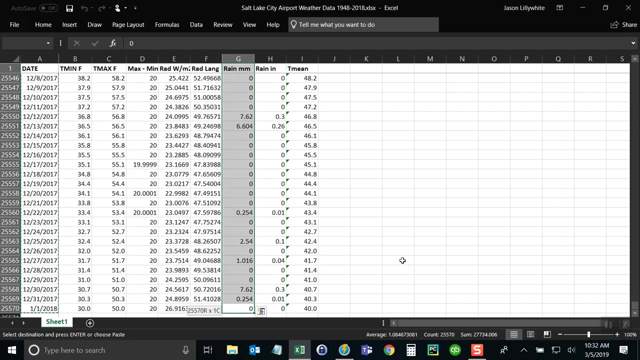 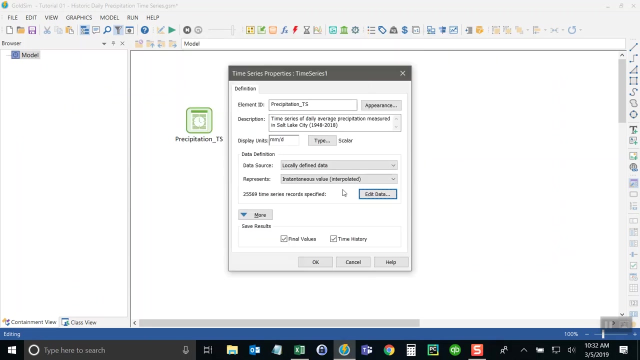 elapsed days format. okay, so I'm going back over to the excel file and I'm just going to select the entire column a of date Apes. copy went back over to Colson paste. now I need to do the same thing for that column. that's this one here. copy paste now when I say okay, goals and we'll walk. 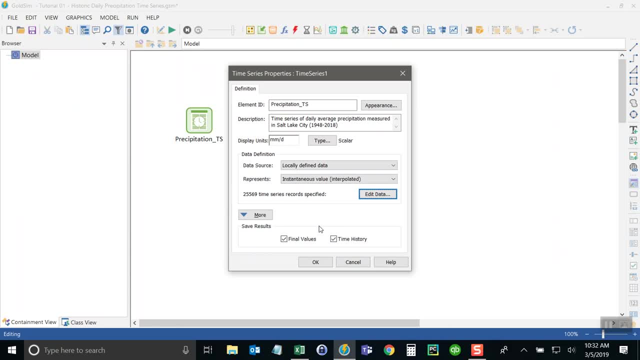 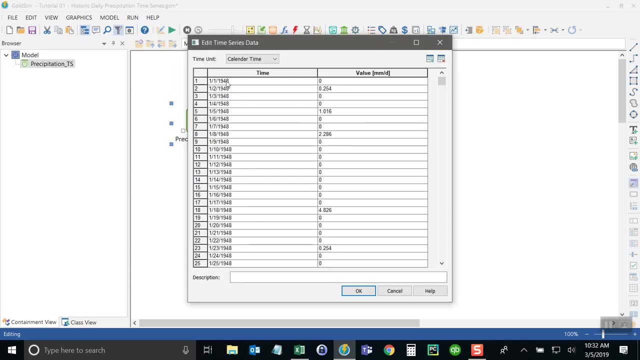 through the entire set and make sure that it's got values in every row and it does, then I click OK. so, as you see, in the time series, if I go back here, look at the dates, it's January 1 1948 through January 1 2018. so now I can come up here to the 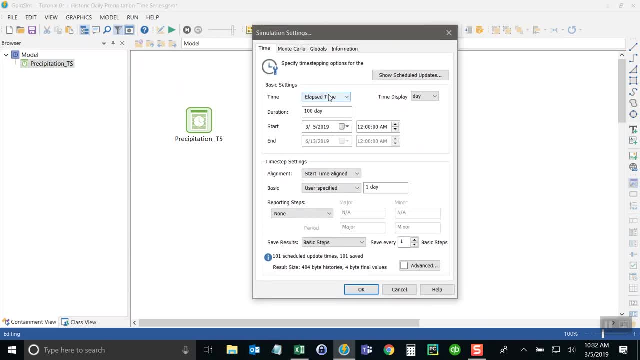 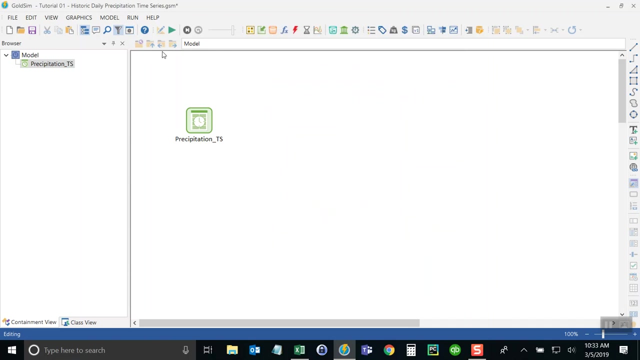 simulation settings of the model, and I'm going to change the time format to calendar time, change the start date to 1 1 1948 and 1 2 6 one 2018, and then i'll keep this as a one day time step. say: okay, now i can run the model. 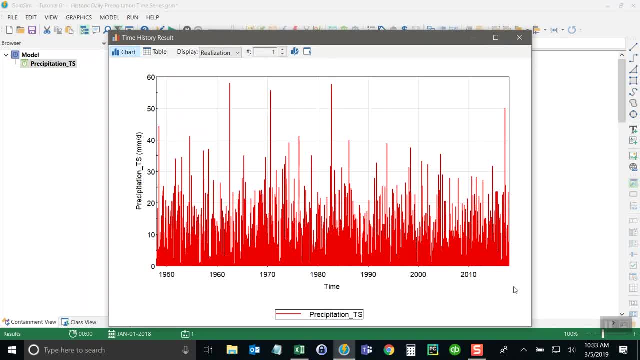 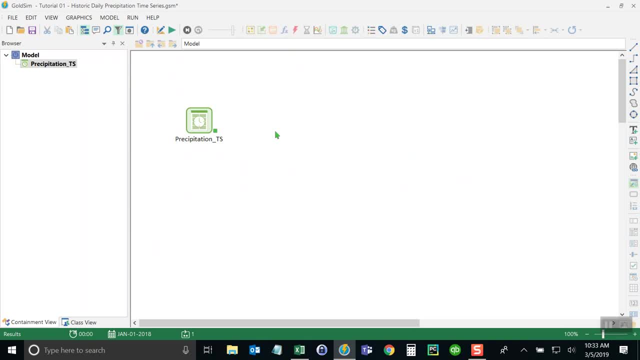 right click on the element and look at the time history, and it shows me a plot for all of those years. now our model is ready to be using precipitation data. but before we end the tutorial, i want to show you one more thing that you can do with gold sim, and that is to run a. 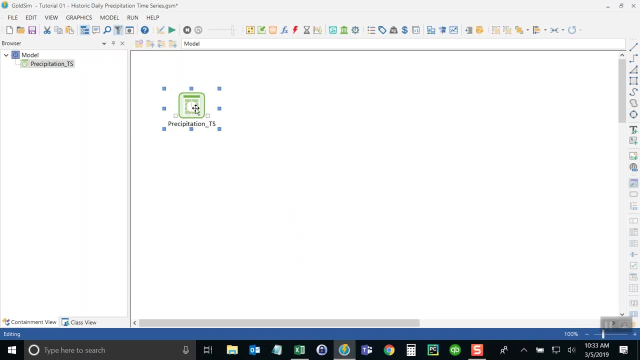 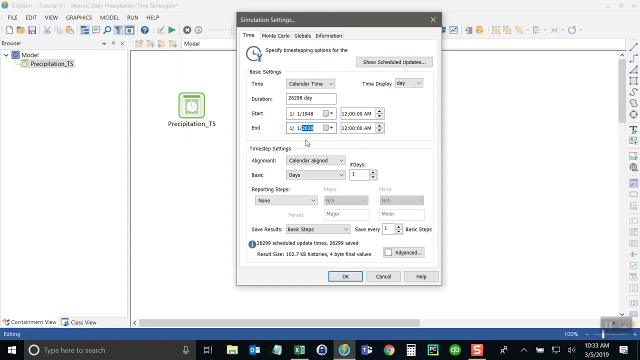 monte carlo simulation that samples the years randomly in our time series. so let's say that we want to do a future simulation for just a single year in the future. so i'll change the simulation settings to run for just one year in the future. so we'll say it's running from. 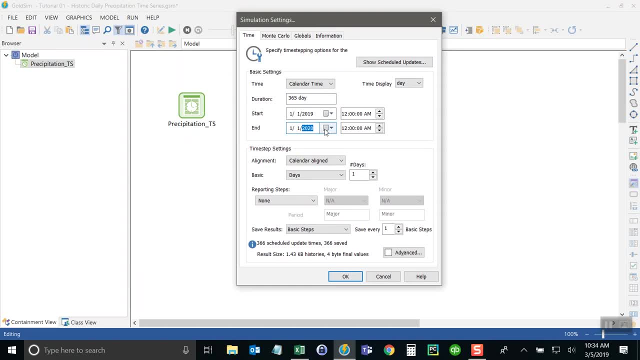 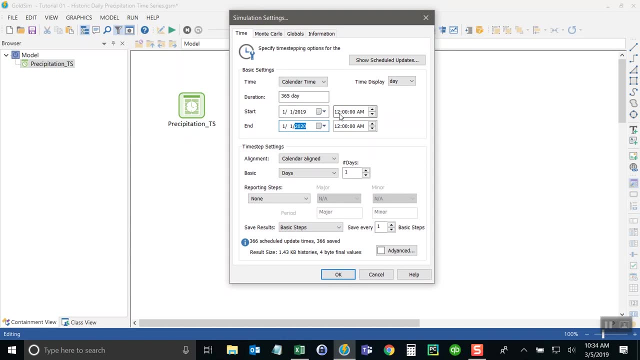 january 1 2019 through january 1 2020, well as of the date of this, of this tutorial. when i'm doing it right now, it's um partially in the past and partially in the future, but we'll just assume this is a. 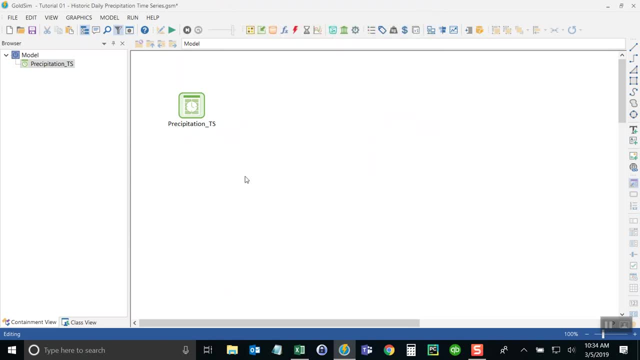 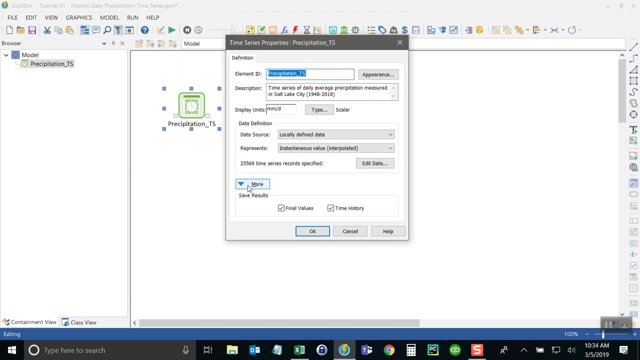 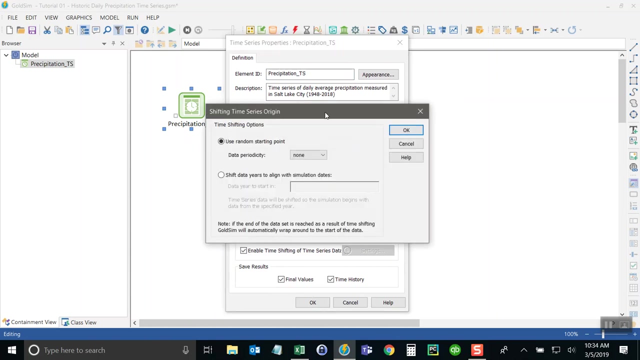 future simulation and you want to run it for a single year now in order to sample our historic data set. we need to go to the properties here and and then click on this more button for the advanced properties and then select what's called enable time shifting, and what this allows you to do is 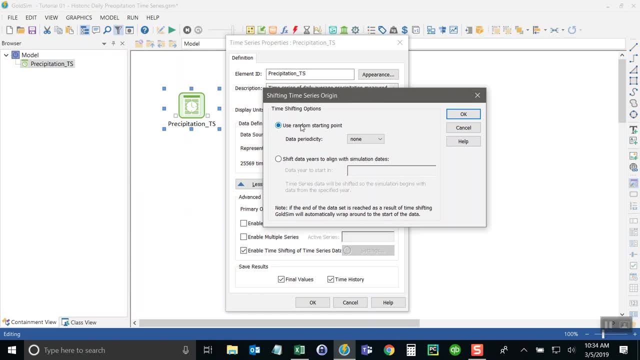 go into the time series and sampling it at random or sequentially. for now we'll just randomly sample the timing, the time series, on an annual basis. so what that means is we can run many future one-year simulations and on each realization of this one-year period, colson will go through and pick a random starting point on january 1 for any random year in the. 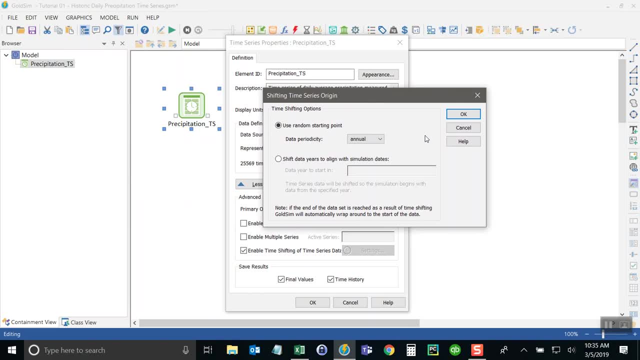 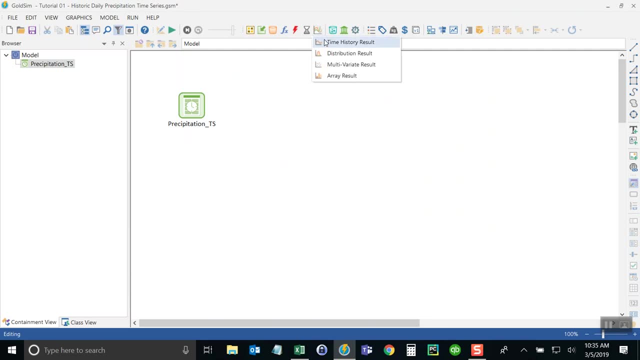 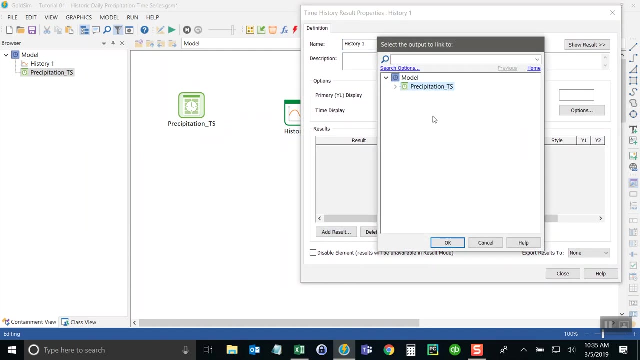 simulator in the in the future time series. now, with that done, we need to create a permanent time history chart so that we can visualize the uh, the results here. so i'm just going to now add the precipitation output so that it's put there. we can change the. 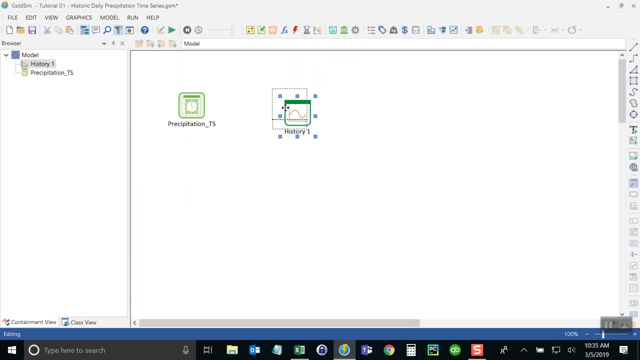 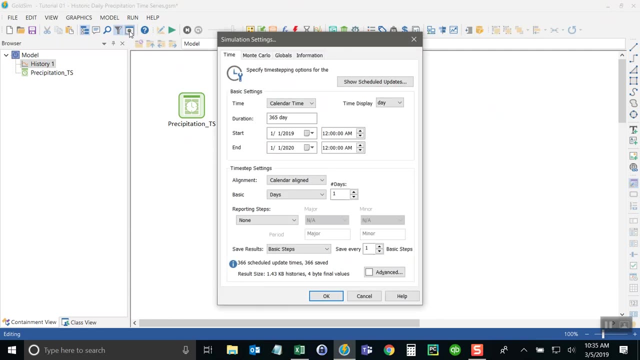 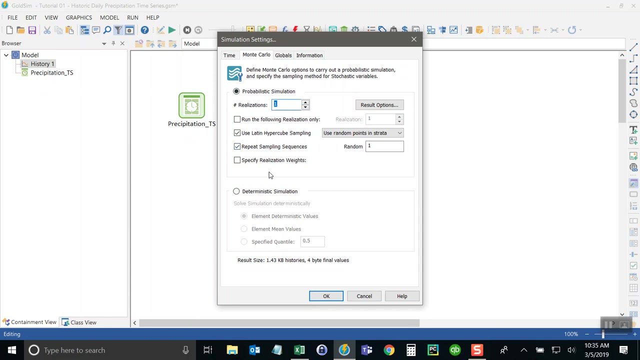 label a little bit there, okay, the other thing i want to do is change the simulation to run as monte carlo, so i'll go back to the simulation settings clicking on the monte carlo tab, and now i'm going to run the simulation for a number of realizations. in this case, i just 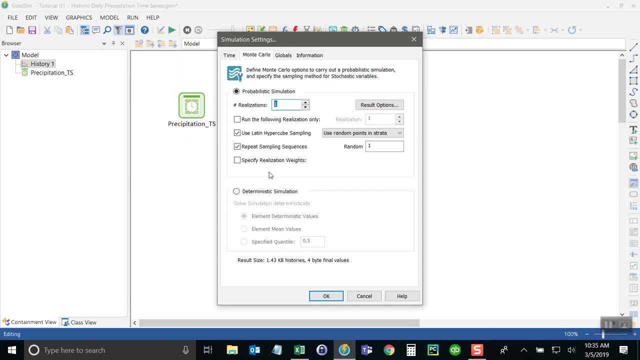 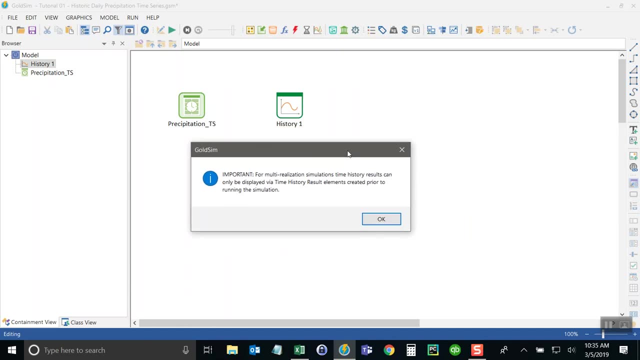 want to run for 70 realizations because i only have 70 years on record in that time series. okay, i get a warning telling me that all the results are not saved unless you attach the results to a time history, which we have done here. okay, so now i run the model and i double click on the chart, and now what we see by default. 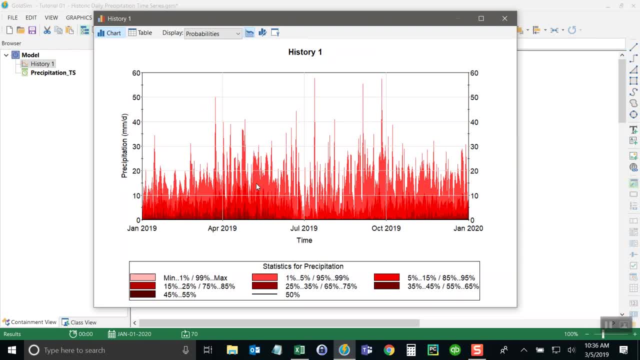 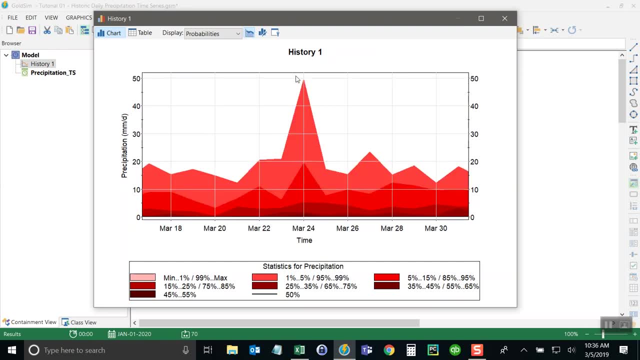 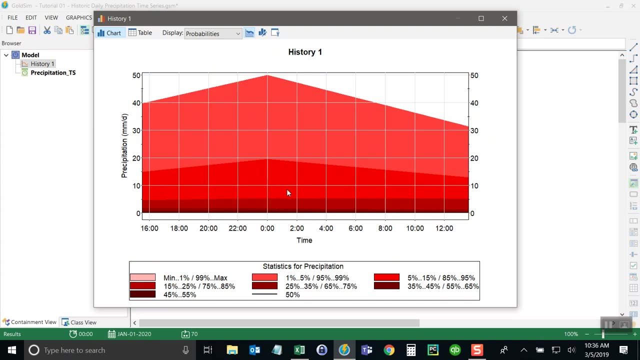 is what's called a percentile chart showing the range of possibilities on any given day. so i could zoom in, for example, on a particular day and i could see that it based on the color coding down here that there are different percentiles possibilities of rain for that. 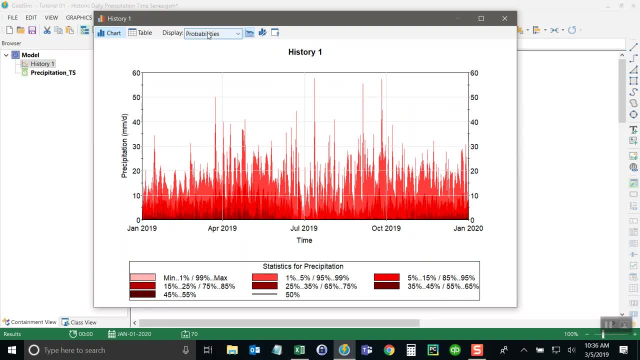 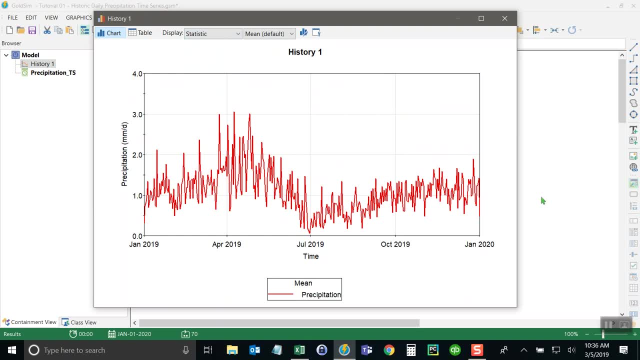 given point in time so i could move around the chart on campus. this via the my area, and i could load this area into mind. the other thing i can do is come up here to the display option and select a statistic so i can see the mean rainfall throughout the year.